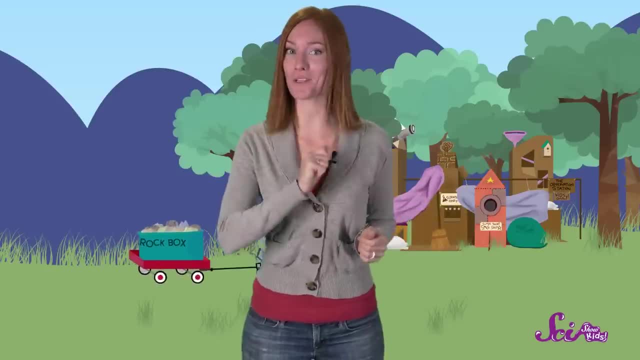 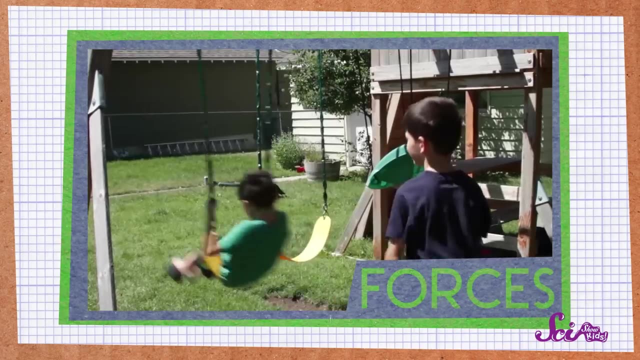 We solved the problem, But how do wheels and axles help us to do work? It all comes down to how much force we need to move the box. We've talked about forces before. They're the pushes and pulls that things put on each other. 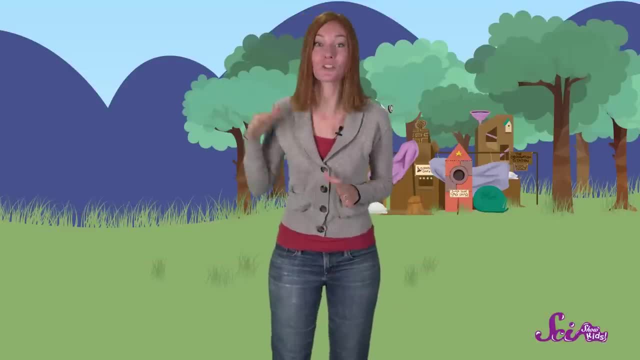 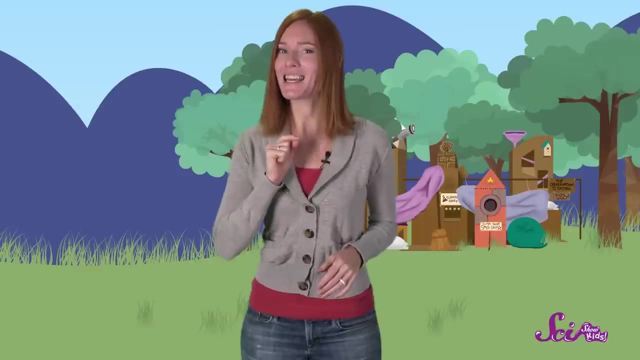 In this case, the force we're concerned with is the one we use to pull on the box. When the box was on the ground, Squeaks tried to put a big force on the box to pull it, But even though he pulled really hard, he could only move it a little bit. 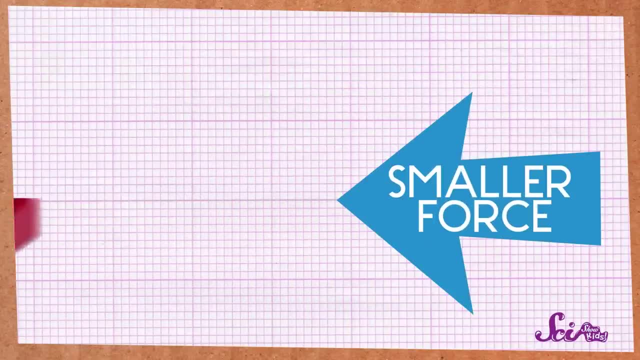 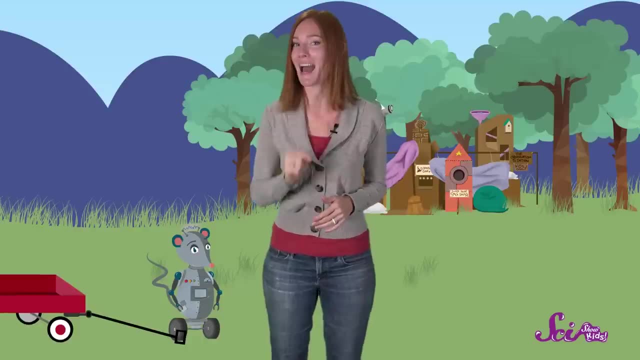 But when the box was in the wagon, Squeaks was able to pull it all by himself easily, So it took less force to move the box, And that's what this simple machine does. A wheel and axle changes how much force we need to move something. 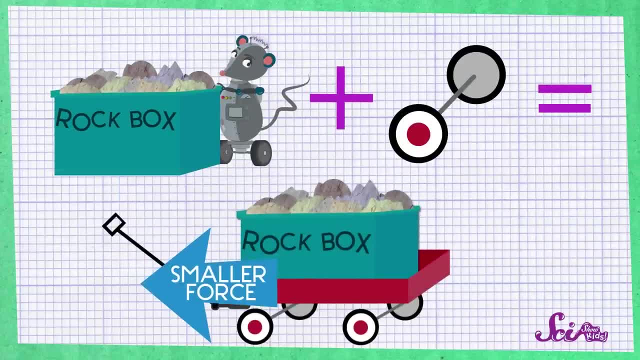 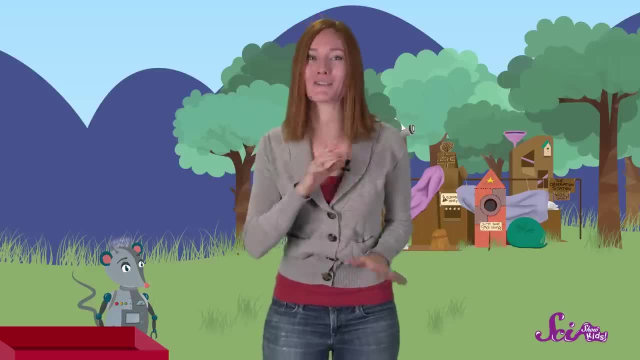 Instead of a big push or pull we can use a much smaller one, And smaller pushes and pulls mean less work for us, Because it takes less force to move heavy things. wheels and axles make it easier to move something a long way. 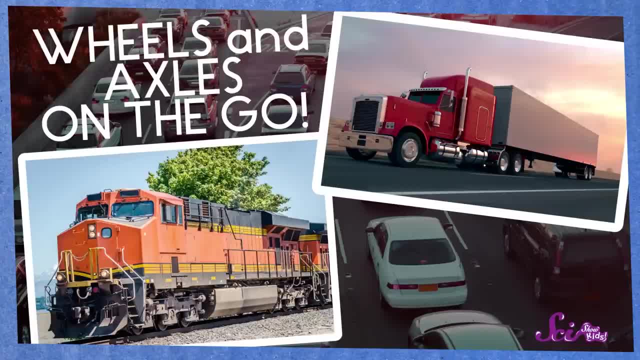 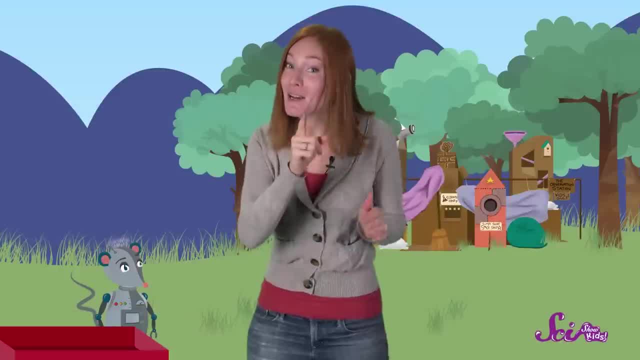 That's why they're part of so many things that help us stay on the go, And that's why you'll see wheels and axles on buses, scooters, wheelchairs and even robot rats, But Squeaks is one robot rat that's earned a break. 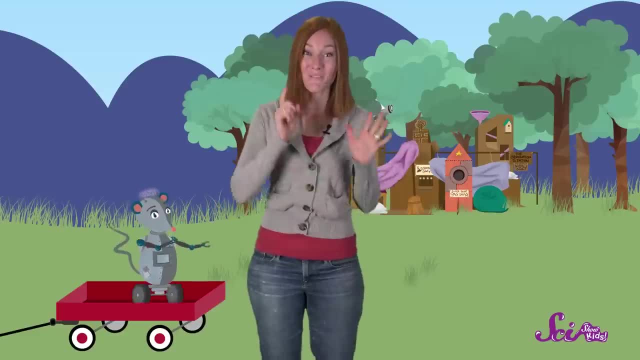 Hop in Squeaks, I'll give you a ride back to the fort. Thanks for joining us. If you have questions about machines or forces or anything at all, just grab a grown-up and let us know in the comments below. Or send us an email to kids at thescishowcom and we'll see you next time.